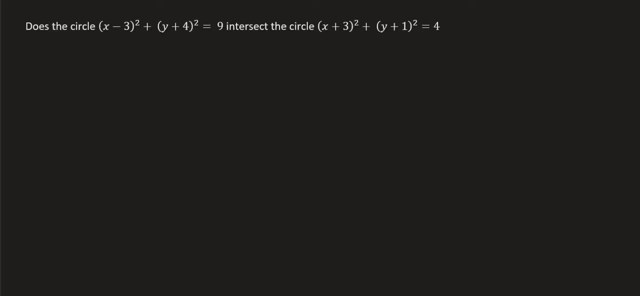 few simple concepts you're going to need to know to approach a question like this. So let's say we've got two circles, okay, so there's circle one and there's circle two. These two circles are not intersecting. Now, mathematically, what that means is the following: If you had to work out, or if you 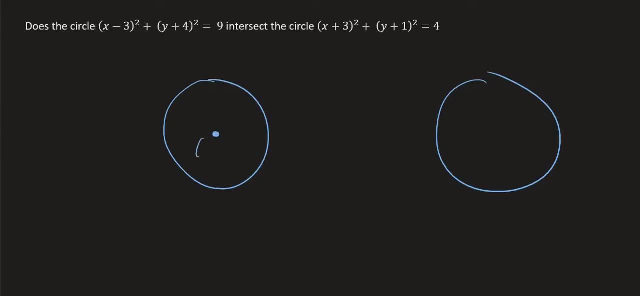 knew the center point of this, this circle here. let's say the center was three and eight and this center was seven and twelve. What you could do is you could work out the distance between those two centers, And let's say that answer was 20.. Okay, so that's the distance between those two points. 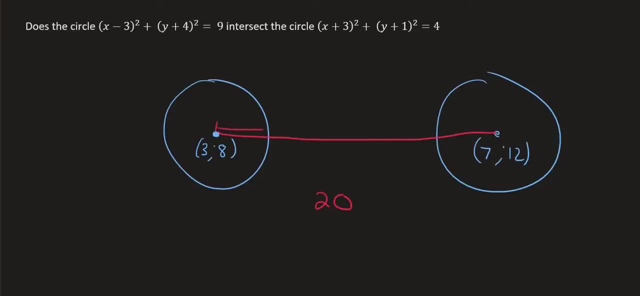 You could then look at the radius of the circle on the left and let's say that answer was three, and then you could look at the radius of the circle on the right and that answer could be five. Then you would see that because the radii, when you add them together, that's eight. That is not. 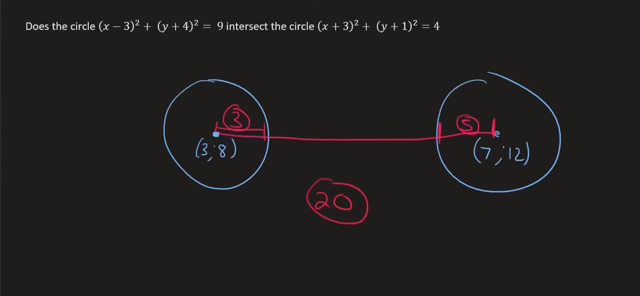 enough to be able to overcome that distance over there. Okay, so the distance between the circles is greater than the length of the two radii, So the circles won't reach each other. Let me show you a different scenario. So here we have two circles that have intersected, So let's see how this would. 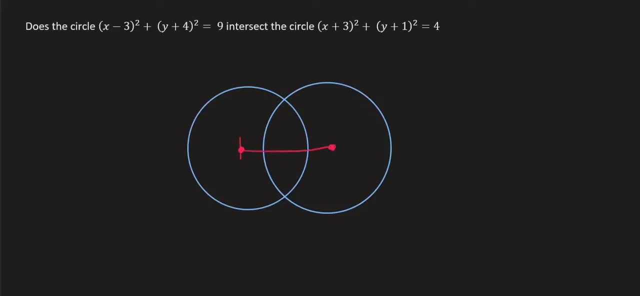 work mathematically. You would work out the distance between their two centers, and let's say that answer was 20. again, You could then work out the radius of the first circle, and let's say that answer was 12.. And then you could work out the radius of the second circle, And then you could. 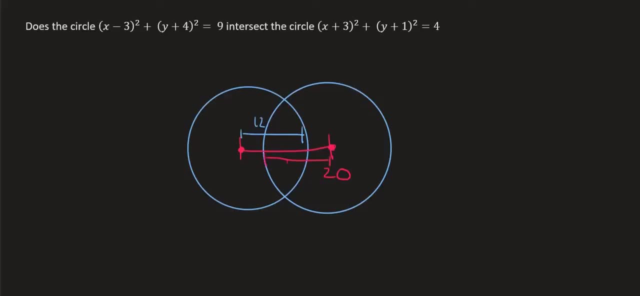 work out the radius of the third circle, which would be from there to there, And let's say that that answer was 15.. So together the two radii add up to 27, but the distance between the two circles is 20.. So of course the two circles would reach each other, because the distance between their 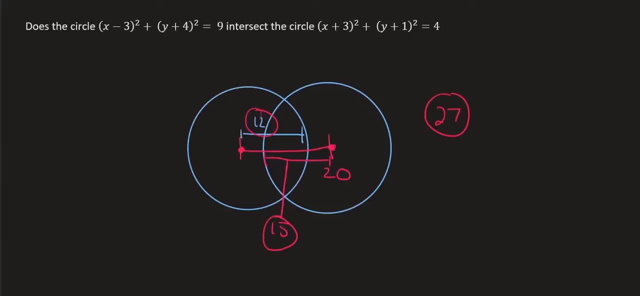 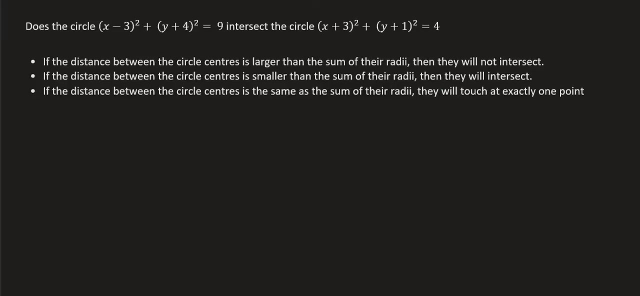 centers is 20.. But if you add the two radii together you get 27.. So the radii are long enough to be able to connect the two circles. So I hope that makes sense. So let's look at the results. So in summary, so here we have it. If the distance between the circle centers is larger, 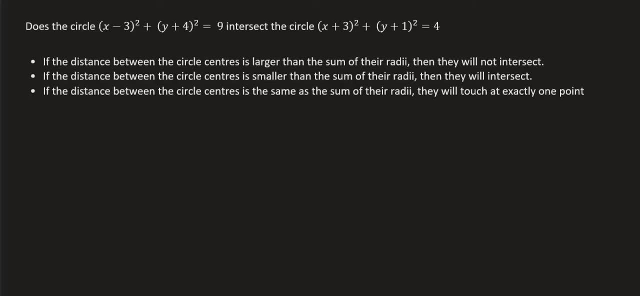 than the sum of their radii, then they will not intersect. Number two: if the distance between the circle centers is smaller than the sum of their radii, then they will intersect, And if the distance- and this is a third one that I didn't show you guys, but if the distance between the 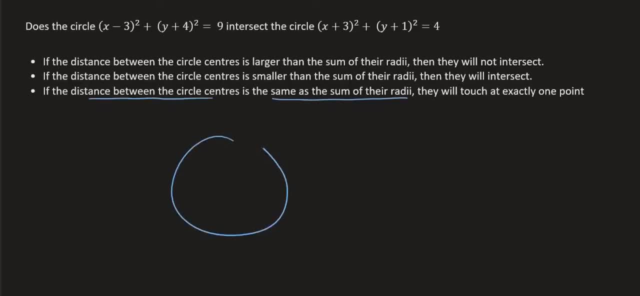 circle centers is the same as the radii, then it looks like this: Then they will touch the center at exactly one point. So if you have the distance, if you have their centers, and the distance between those two is 10, and this one's radius is 3, and this one's radius is 7,, then they 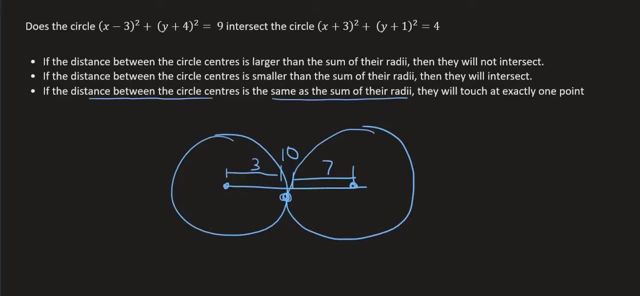 will just meet each other, but they won't intersect like that. Okay, so let's try an example. So in this question we've been given two circles, so we don't need to draw them out, We just need to know what their centers are. So this one, the first one's center, is 3 minus 2.. So we don't need to. 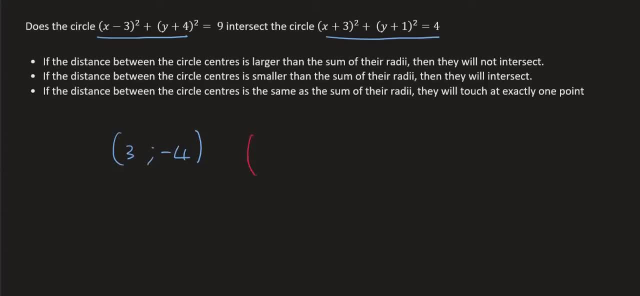 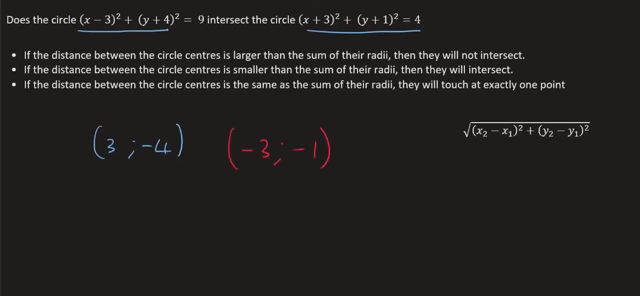 and the other one's center is minus 3 and minus 1.. So we can use the distance formula to work out the length between them. So I'm going to start off with this as 0.2.. So that would look like 3 minus. 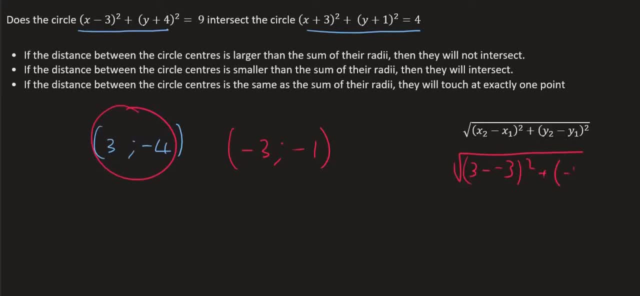 minus 3 plus minus 4 minus minus 1.. And if you type all of that in on the calculator, it gives us an answer of 6.75.. So that is the distance between the two circle centers. I now need to look at the radius of each. 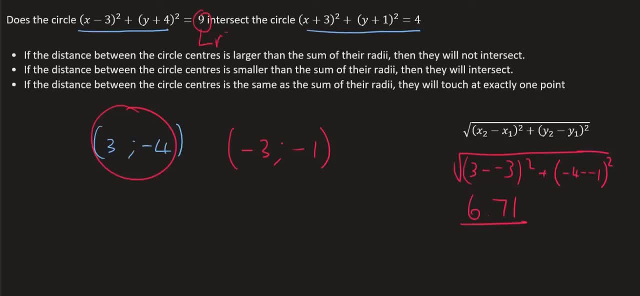 one. So this one's radius is 3, because, remember, that represents r, squared, and this radius is 2.. So if you add their two radii together, which is 3 plus 2, you get 5.. So these two circles are not. 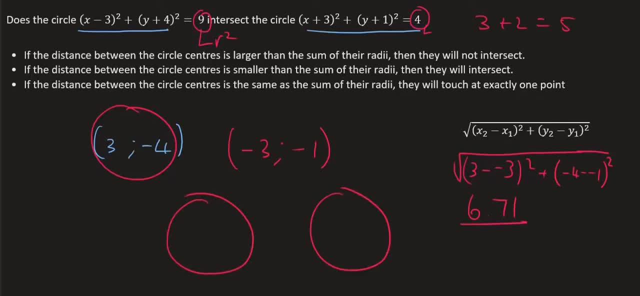 going to intersect because the distance between their centers is 6.71.. But if you add this distance, which is only 6.71, you get 5.71.. So that's the distance between the two circles, So that's the. 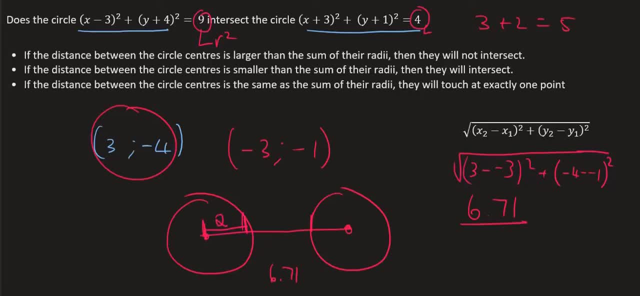 only 2.. And you add this one's distance, which is only 3,, you can see that they will not add up to become more than 6.71.. So they won't reach each other. Let's try another one. So the center.